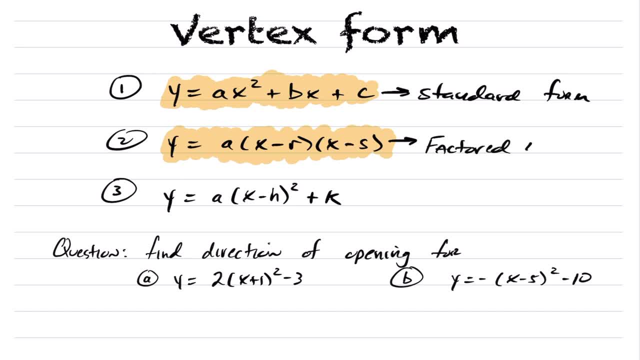 This form is known as factored form. So if you're given a quadratic and you use difference of squares, decomposition, GCF, etc. you're putting that quadratic in factored form And lastly- and this is the form we're going to be focusing on in this lesson- 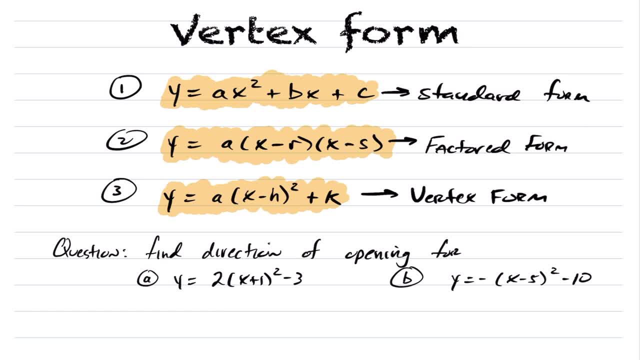 is vertex form. Each of these forms has their own advantages and they give you characteristics about your quadratic that you need to graph the quadratic and understand it. For instance, standard form is going to give you the y-intercept very easily and we'll talk about that in a later. 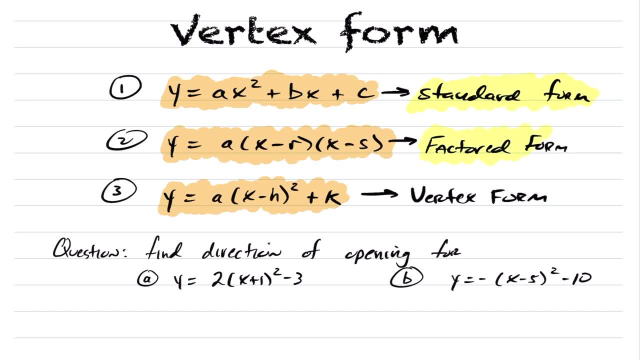 video. Likewise, factored form is going to give you the roots. And lastly, vertex form. you guessed, it gives you the vertex of your quadratic. All three of these forms actually give you the direction of opening. and again we'll talk about 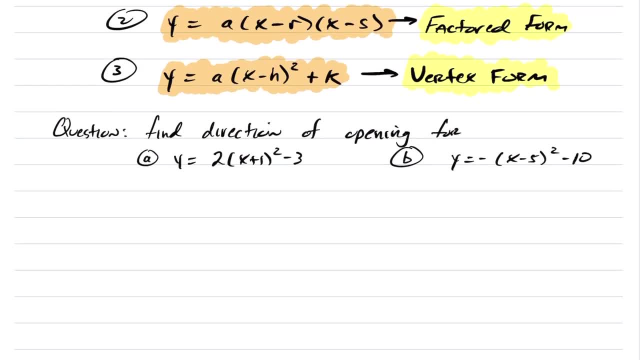 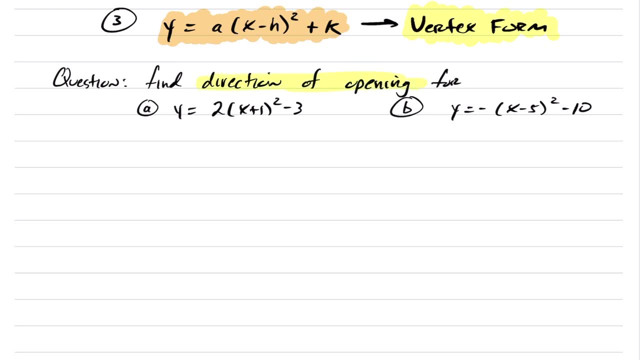 that Okay. let's take a look first at this idea of the direction of opening of your quadratic. How can you figure out if your quadratic is opening up or opening down, Where you look to decide? that is in the description below. So if you're going to look at this idea of the direction, 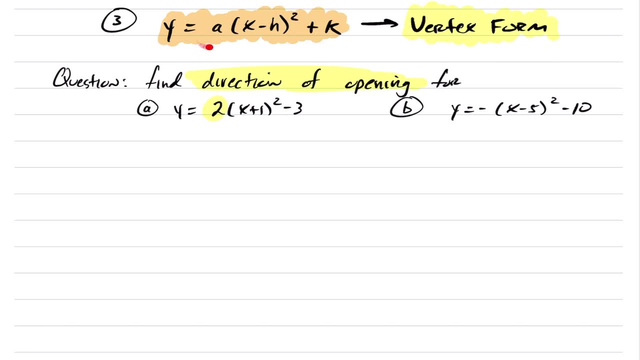 of opening of your quadratic. how can you figure out if your quadratic is opening up or opening down? How can you figure out if your quadratic is opening up or opening down? Where you look to decide, that is, you look at the a value. Notice your a value, for your vertex form is sitting right. 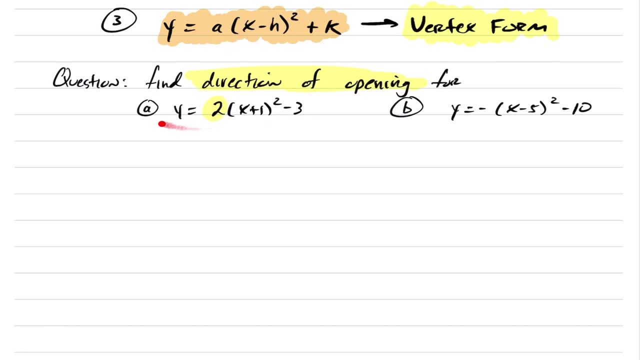 here. This is in vertex form, And because this is in vertex form, I know my a value here is two. If your a value is positive, your quadratic will always open upwards. The reason for that is this expression right here- will always be greater than or equal to zero. Why is that the case? Well, 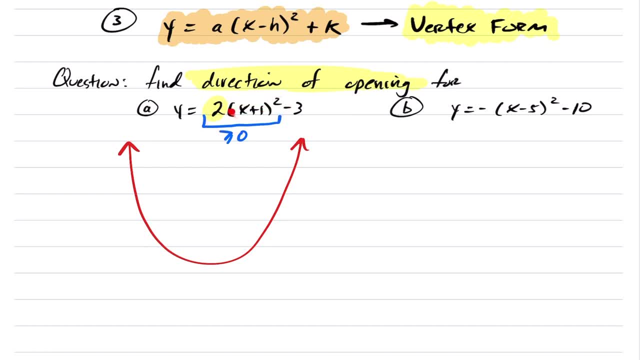 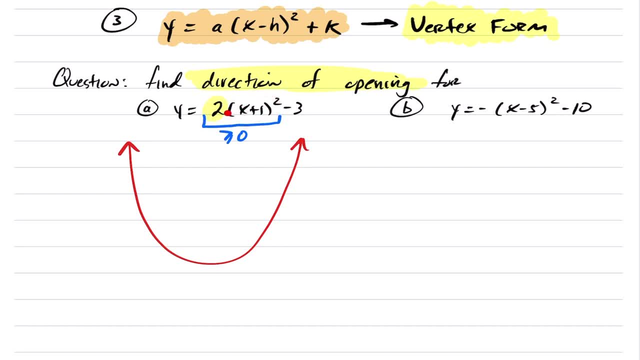 be positive And then you're multiplying by a positive number. So this expression right here, independent of what you let x be, if you let x be negative 100, or let x be positive a million, no matter what you do, this term right here will always be greater than or equal to zero. 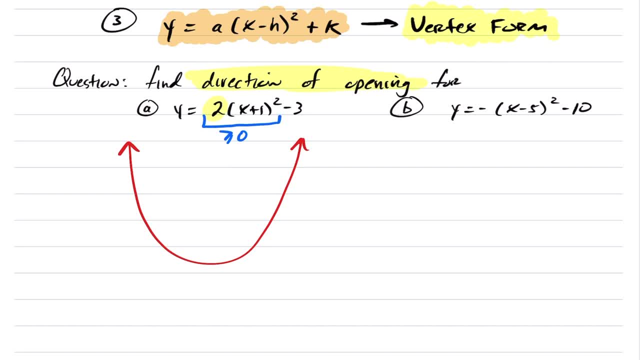 So that means that as I choose values that are further and further to the right and left of my quadratic, this will get larger and larger and larger, For example here: take a look here. Suppose I were to let x equal two. If I let x equal two here we'd have y equals two. 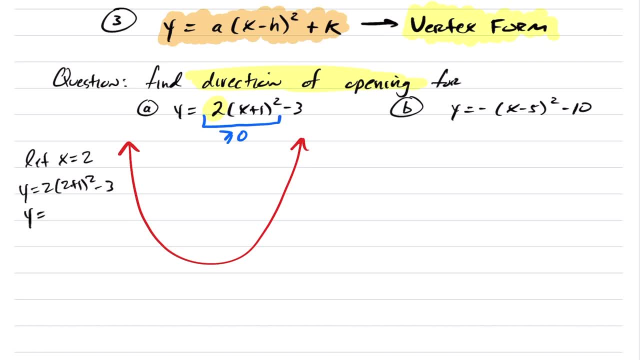 two plus one squared minus three, y would be two times three squared minus three, And then we'd have 18 minus three is 15.. Okay, so that means that the point 215 is on my graph. But what would happen if I let x be 20?? So now we're going further. 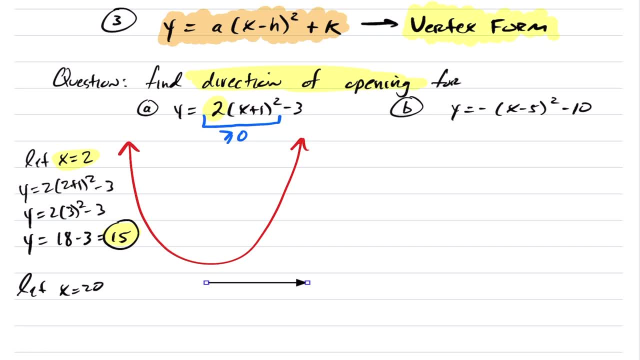 to the right of my quadratic, what happens? So maybe- and again I'm just estimating, maybe. this is the point 215.. Now let's say I let x be 20, what output do you get? Well, you're going to get. 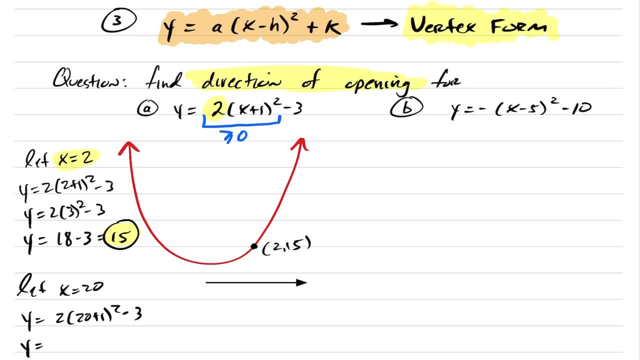 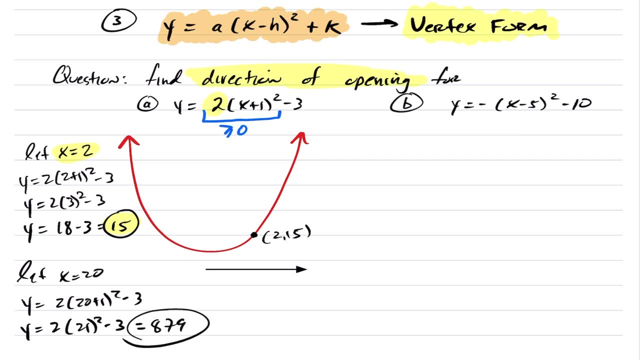 20 plus one squared minus three, And then y is going to equal two times 21 squared minus three. If you calculate that, you'll notice you get, you'll get 879.. So therefore, by going over 20, now we're maybe right, here- we're at the point 20,. 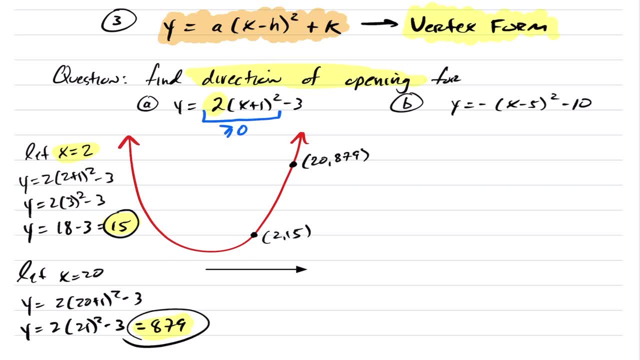 879.. All right, Likewise, had I chosen negative values, going the opposite direction, you would also have very, very large numbers, because again you're squaring that value. Okay, so the direction of this quadratic is all determined by this leading coefficient, a. 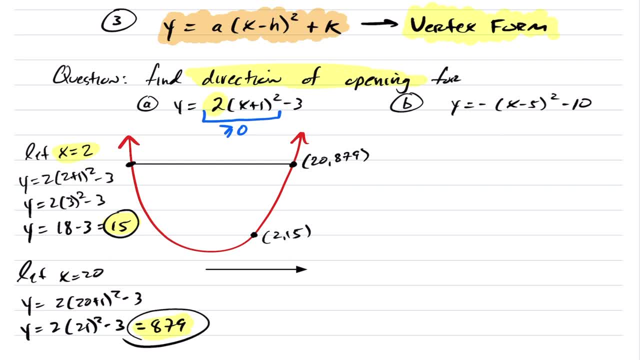 On the other hand- you'll notice with the next example here- my leading coefficient is a negative one And because of that this quadratic here is always less than or equal to zero. So this is always decreasing. So this quadratic will open downwards And again you can see that with some examples right As I move. 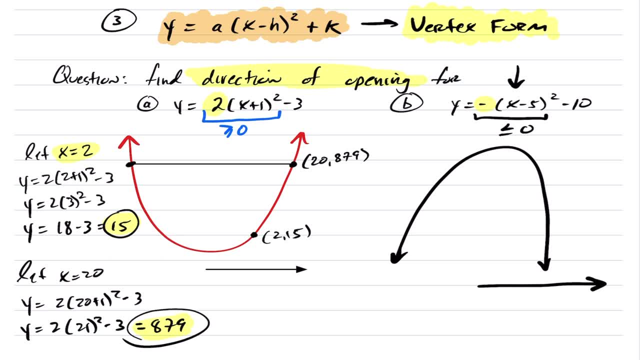 towards the outside of my quadratic and we let- let's say I let- x equal two. this time I'm going to get y equals negative negative two minus five squared minus 10, which case get y equals negative three squared minus 10.. 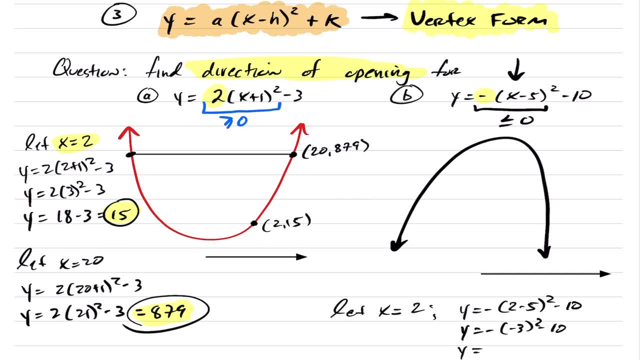 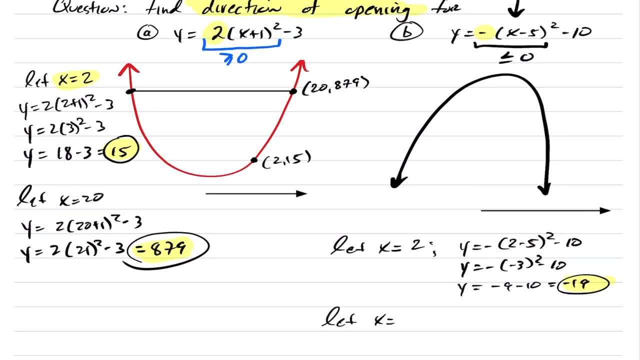 And this becomes- and this becomes negative. nine minus 10 is negative 19.. Okay, now what happens if I let x be 20?? This time we're going to get: y equals negative 20 minus five, squared minus 10.. And that becomes 15.. 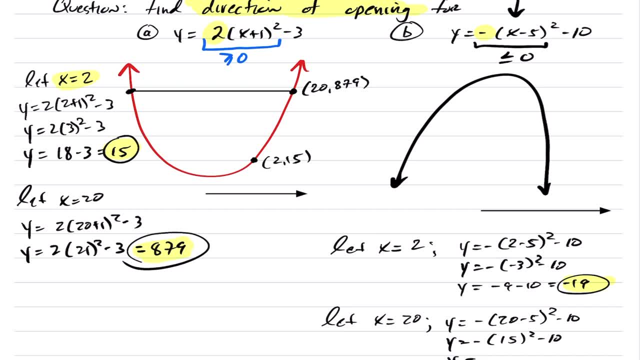 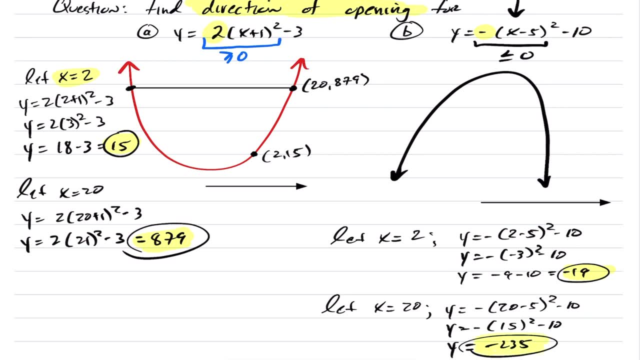 squared minus 10.. And if you calculate this on your calculator you get negative 235.. So again, you can see here as I move towards the right hand side. our first point was the point two, negative 19.. This next point, at 20, was far lower. 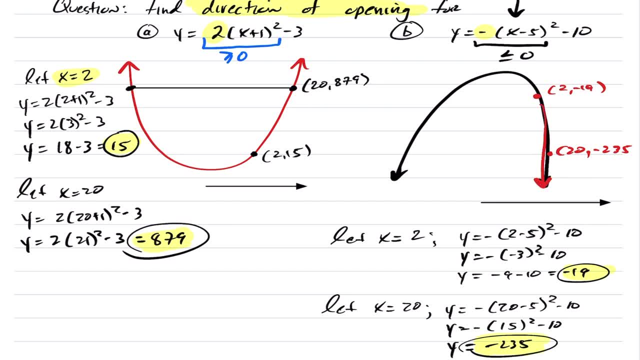 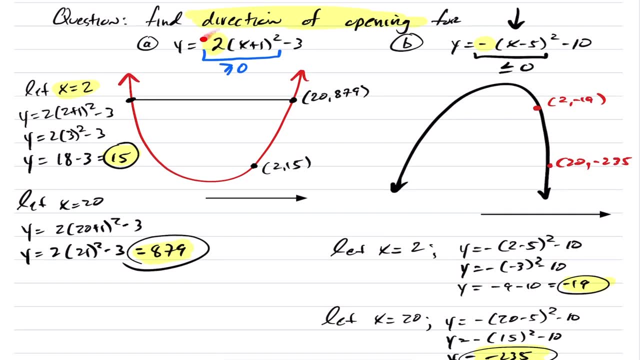 And you can see that direction is being pushed downwards because of that leading coefficient. All right, so to summarize here: if your a value is positive, quadratic opens up. if the a value is negative, quadratic opens down. It's as simple as that, But I thought it was important to understand. 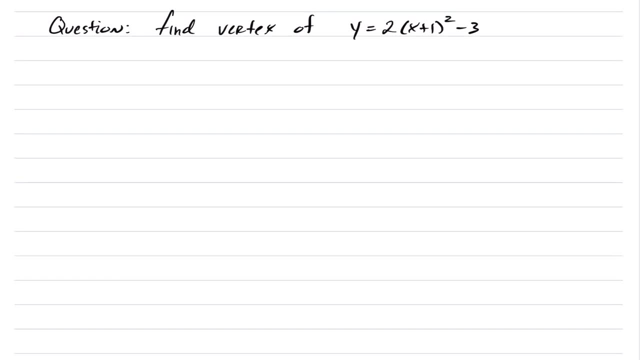 sort of why that is the case. Okay, next thing. here Again I'm in quadratic, I'm in vertex form, I have a quadratic in vertex form. here I have a quadratic. I know that the a value is positive. So, because the a value is positive, I know my quadratic opens up and I know that the a value is positive. 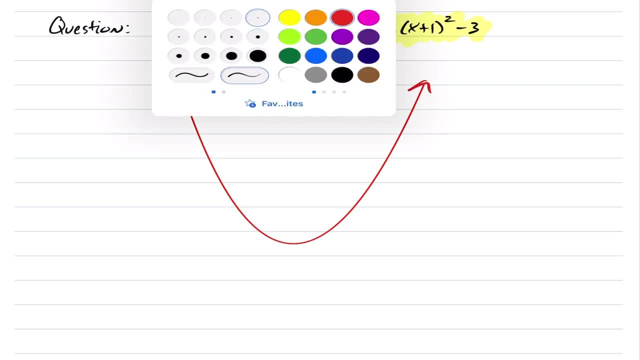 I know that the a value is going on and I know my quadratic opens upwards. If I'm now here, I'm now in parabola, I'm at a straight line. my sort of love line opens upwards. So you know, maybe it looks something like this: 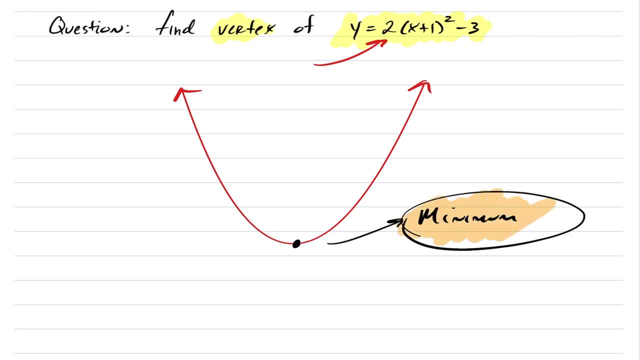 We want to find the vertex, so my vertex is located right here. That point right here is a minimum yard value. That's a minimum value. So the question becomes is: how do we find that minimum point? What is the value of x here? 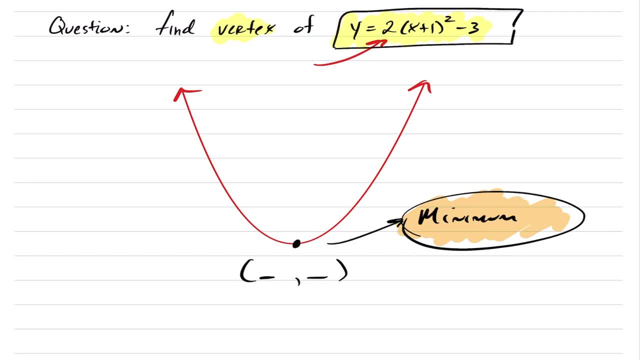 It's behind three points. I can't find the point here, So now I have to find the point in two as possible. again, as we've discussed here, this expression right here will always be greater than or equal to 0, so therefore the smallest I can make this: 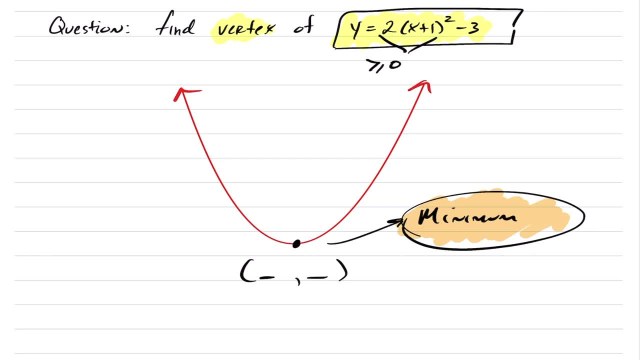 expression is 0. so how do you make this expression 0? you have to let X equal negative 1, because if I let X equal negative 1, what happens here is the inside cancels. any other value you choose will be larger than negative 3. 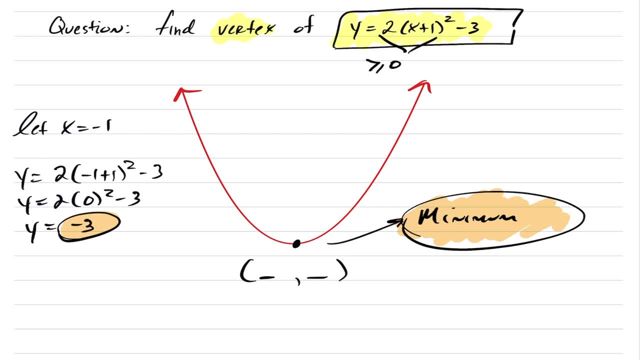 and you can try it out yourself: if you let X be 10, if you let X be 0, 100, negative 100, whatever you do you will, it will give you a larger value than negative 3. so therefore, this point here has an X value of negative 1 and a Y. 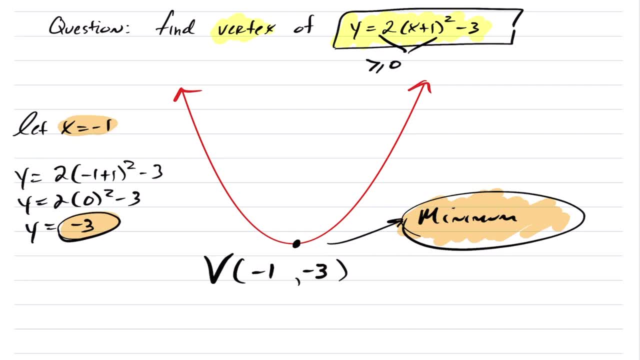 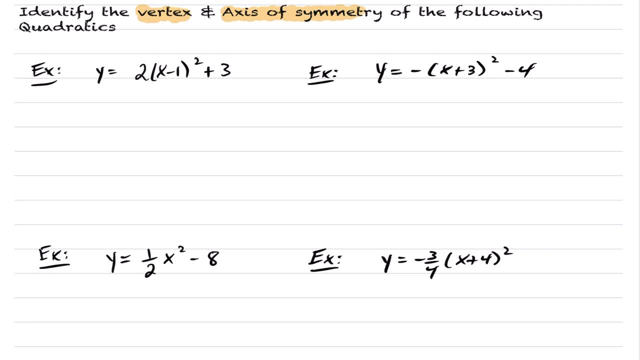 value of 0.. of negative 3, this is my vertex. okay, let's try to apply what we've learned here, try to identify the vertex and while we're at it, we'll also extend our study to talk about the axis of symmetry here. so for our first example here, 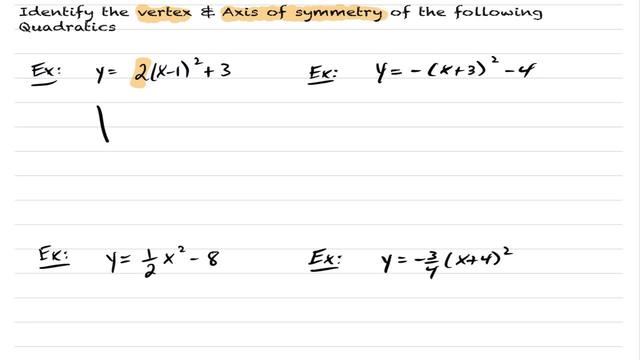 notice here the leading coefficient is 2, so it's positive, so it's going to open upwards. I want to find this point right here. like we said, what you need to do is you need to make the inside value 0, so I have to figure out what value of X will. 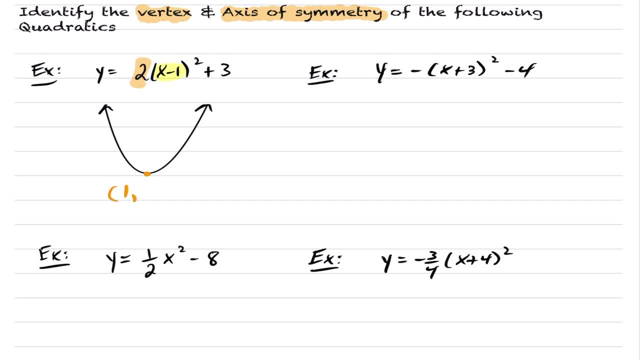 make what's in the brackets here: 0? well, that's going to be 0.. that's just going to be X is 1. but if X is 1- we saw here- the Y value must be 3. so my vertex here is 1- 3. okay, let's try it again for the next one now in this. 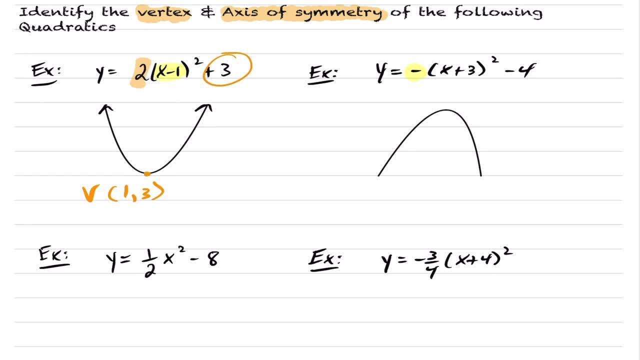 question. the leading coefficient is negative. so now this quadratic opens downwards this time, and I want to be able to find this maximum point here, while you ask yourself the same question: for what value of X will the inside be 0? well, in this case, here it's going to be 0. 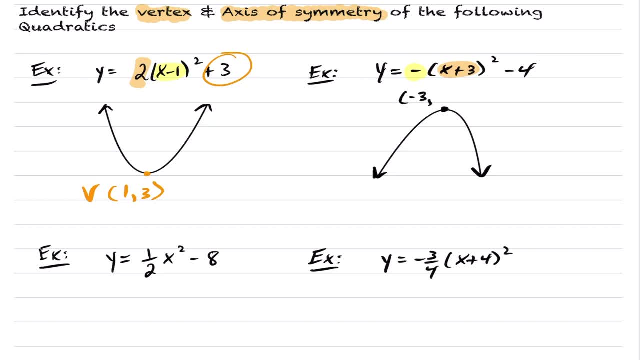 0.. 0. 0.. it's going to be minus 3. what's the corresponding Y value negative 4? so this is my vertex this time. now these questions also ask for the axis of symmetry. your axis of symmetry, like we talked about, is a vertical line that. 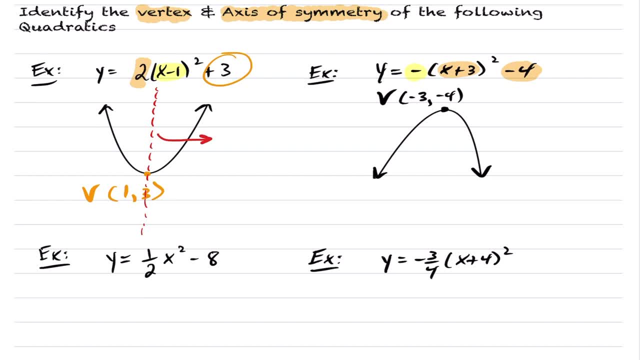 cuts the quadratic into two equal pieces. well, because it's a vertical line, it's going to be: X equals 2. X equals to what you always grab, your X value of your vertex. so this will be: X is 1. likewise, you have a vertical line and you have a. 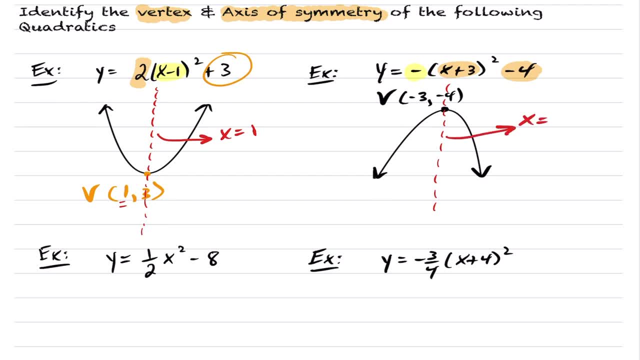 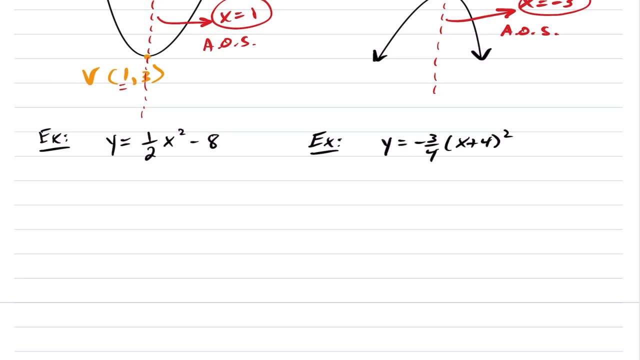 vertical line. vertical lines are always expressed as: X equals 2, X equals to what minus 3, so this is my axis of symmetry. okay, let's continue on now. this is actually in vertex form. we just got to adjust it a bit to make it kind of. 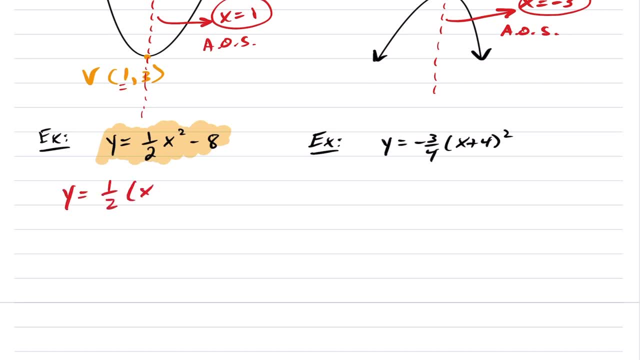 fit the formula for vertex form. so there's my a value. I'm just gonna write an X plus 0, squared minus 8. this still falls under the category of being vertex form. now, in this case, here my a value is positive, so it's going to open. 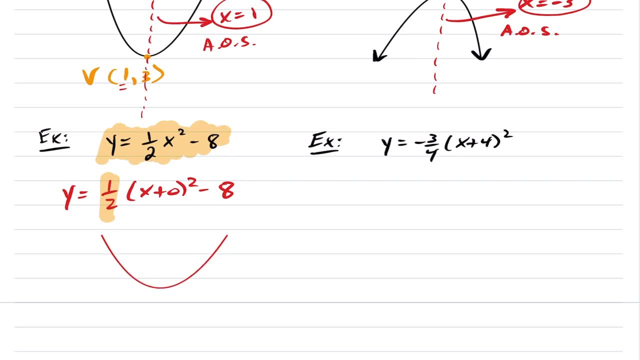 upwards. so we still got our quadratic opening upwards here. I want to go ahead and find my vertex. so what are the coordinates of my vertex here? like we've always talked about here, you want to make this the opposite. so how do I? what value of X will make the inside zero? that'll be, X is 0. this value right here. 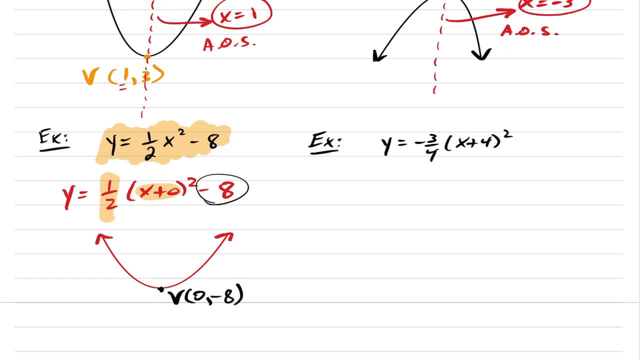 is my y-coordinate, so my vertex here is 0 negative 8. the axis symmetry is a vertical line. it's going to cut the quadratic into two equal pieces. because it's vertical line. it's going to equals to x, equals to what it's always going to be- x equals to your x coordinate. so in this case, 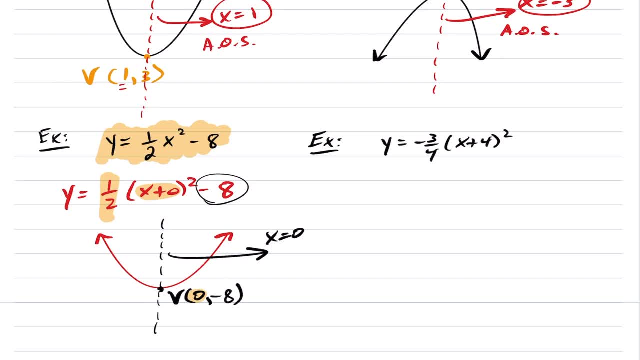 here. this is x is zero. okay, let's continue on my next. my next quadratic here is in vertex form. leading coefficient is negative, so it's going to open downwards this time, and now i want to go ahead and find the vertex. well, again, ask yourself the question: for what value of x will the inside? 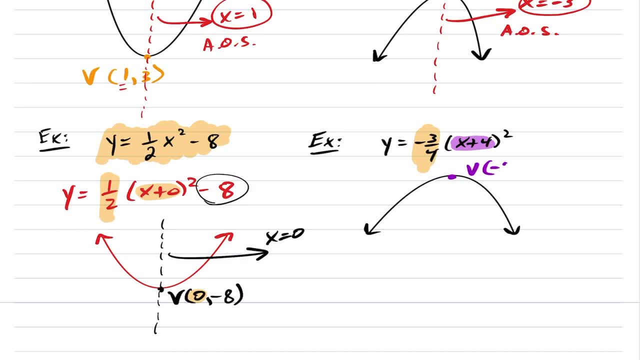 be zero. well, the inside is going to be zero. when x is negative four this time, what's corresponding y value? we have nothing written here- must be a plus zero at the end. so my vertex will be negative four, zero. draw yourself a vertical line. therefore, my axis symmetry is going to be: x equals two. 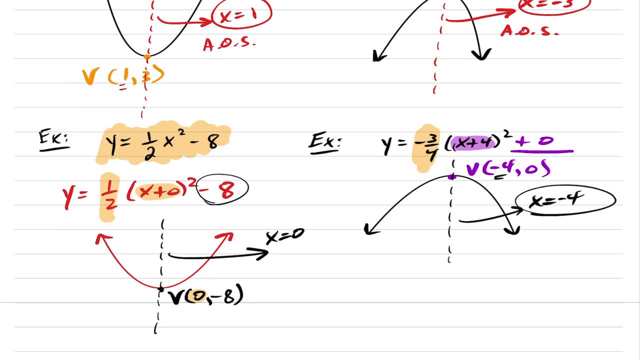 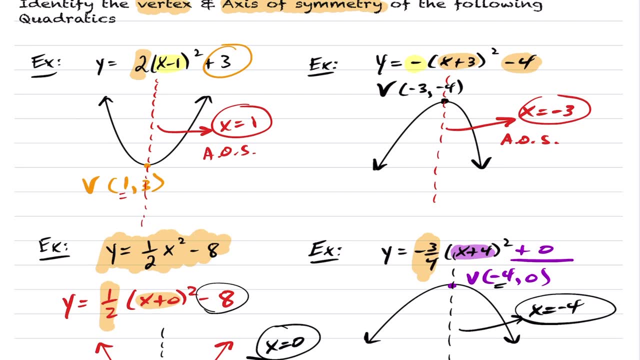 you just grab your x coordinate of your vertex and that'll be negative four. okay, that concludes this lesson. uh, introduction to given a quadratic in vertex form. how do you find the vertex, how do you find the axis of symmetry and how do you know the direction of opening?